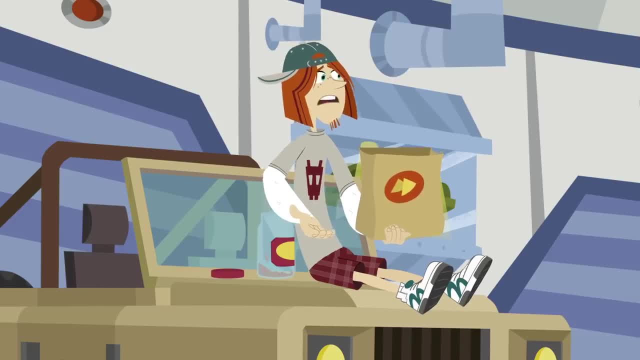 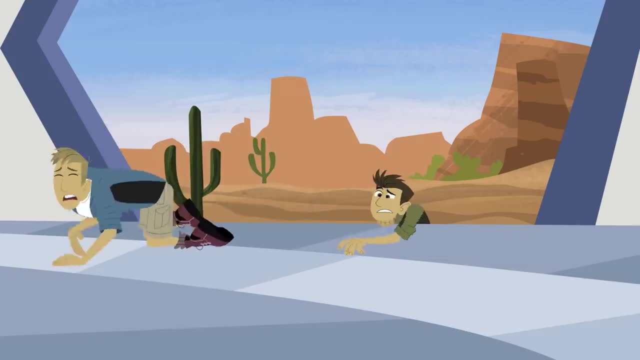 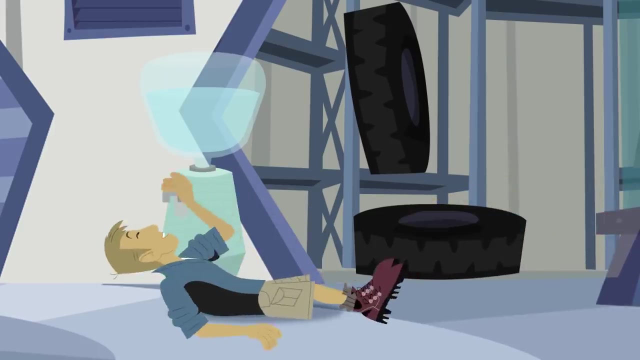 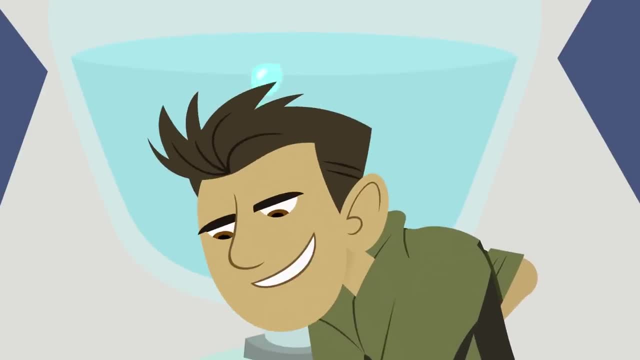 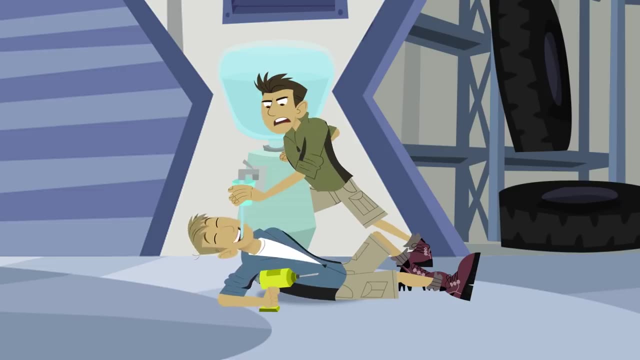 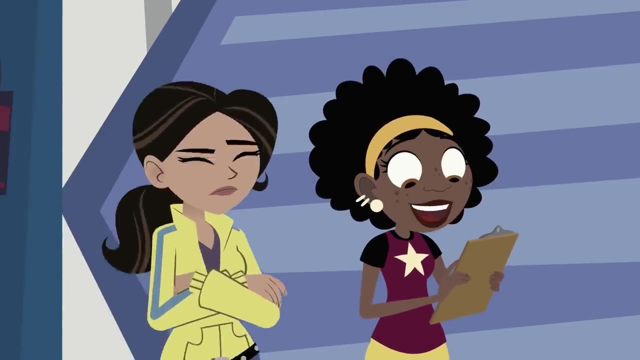 Hey, Hey, Hey Hey, Let me air this up a little bit. I gotcha, Huh, Oh, Oh, Oh, Oh, Oh, Oh, Oh, Guys, knock it off. We have to conserve. This is our last bottle of water. 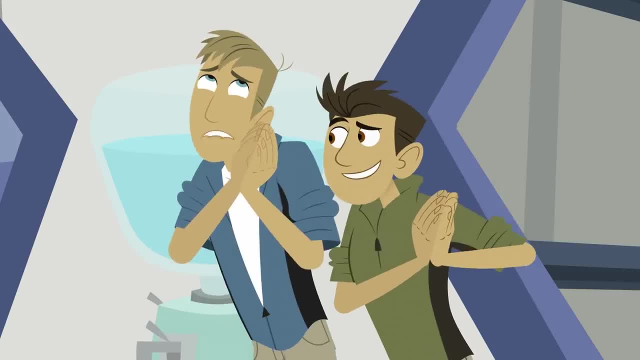 Aviva and I have just decided we have to leave now and go to town and get resupplied- What? But we just got here to the Sonoran Desert and we've only met a few of the creatures who live here. 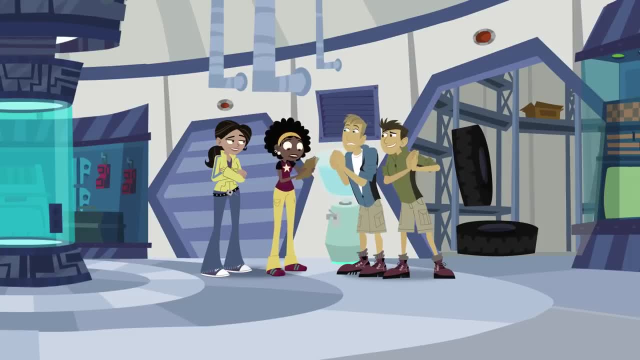 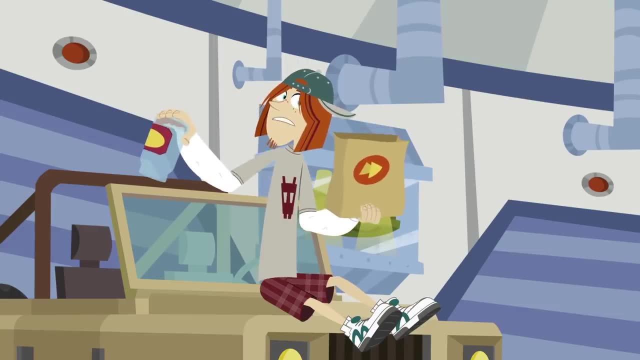 I told you: I know, but we've run out of so many things, They're going away. Oh no, This is the last bag of nachos and we have no more salsa. Oh yeah, you do have to have salsa for your nachos. 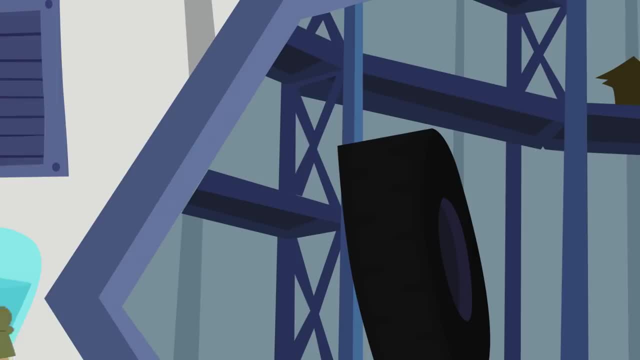 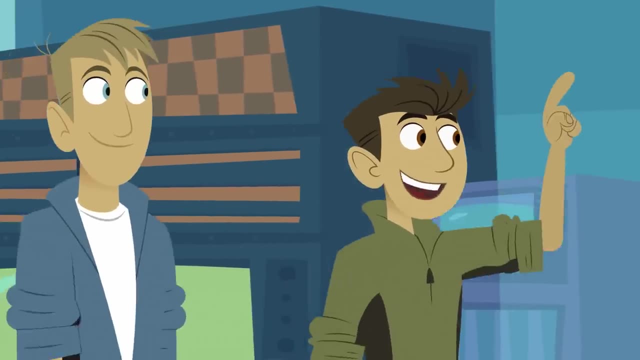 especially when you're adventuring the desert southwest. Wait a second, We can't go now. We're just on the tail of that speedy little mystery lizard over there. Leaving now is against the Wild Kratts, Creature Adventure and Code of Conduct. Yeah, you're right bro. 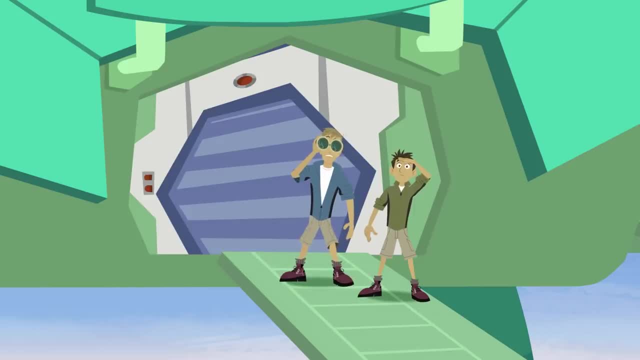 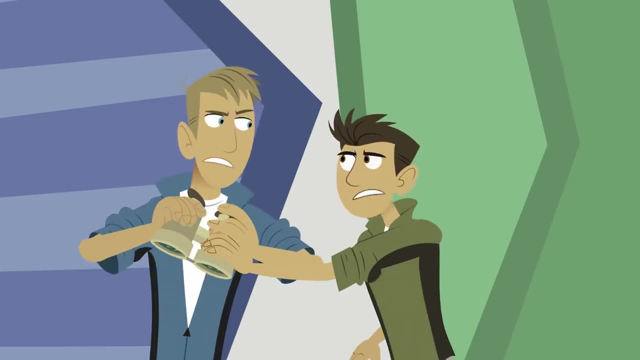 We've got to stay until we know exactly who that mystery lizard is. Whoever it is, it'll be a new animal for our life list. Well, seeing through binoculars doesn't count. We have to see it up close and personal to add it to our life list. 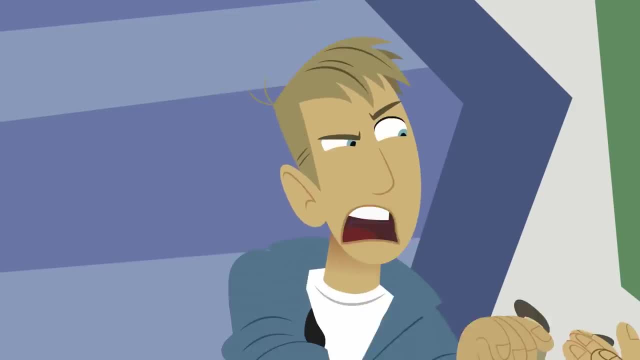 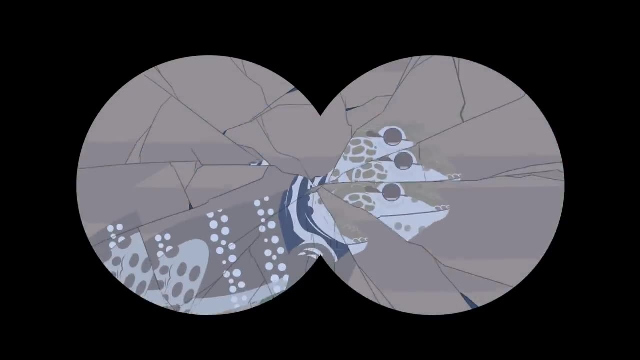 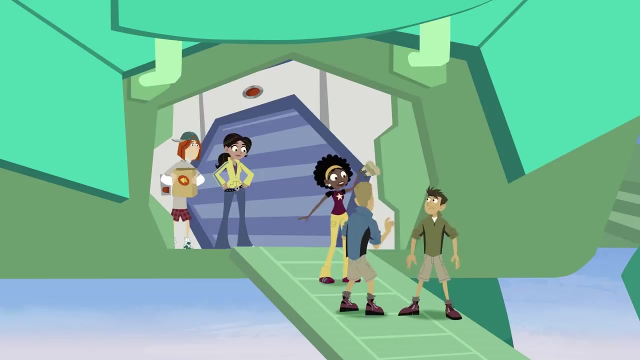 I know, but at least we know what we're trying to get a closer look at. Oops Whoa, It has two tails, three eyes and, uh Martin, The binoculars are broken. Now we have another reason to head to the nearest town. 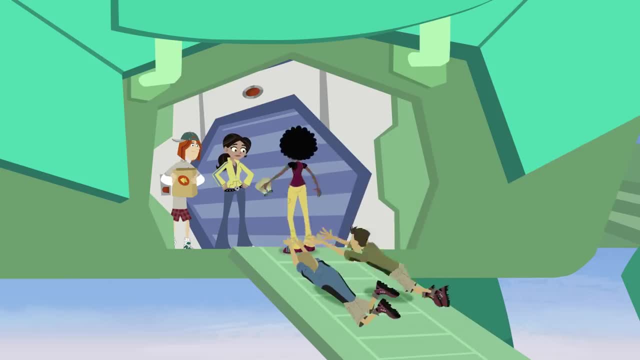 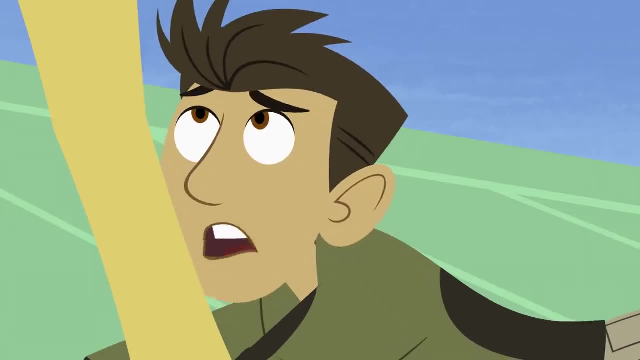 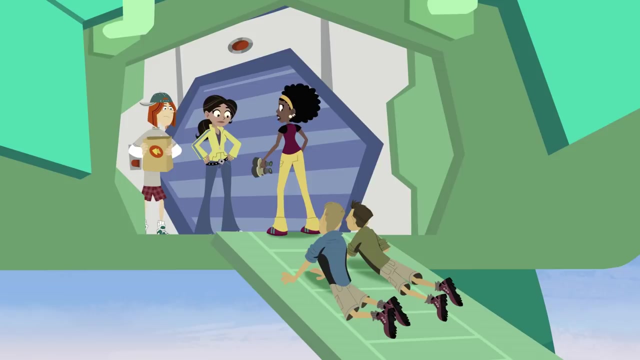 New binoculars. Come on, guys, get packed up and ready to go. Please. just five more minutes. Oh, come on. we just have to get close to that speedy mystery lizard. Just five more minutes, please? Fine, I still have to realign the Tortuga's hover thrusters before we take off. 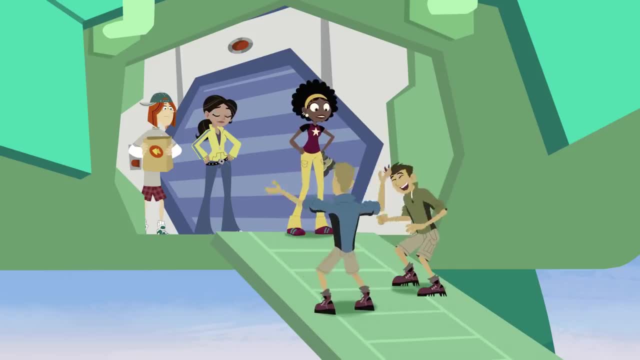 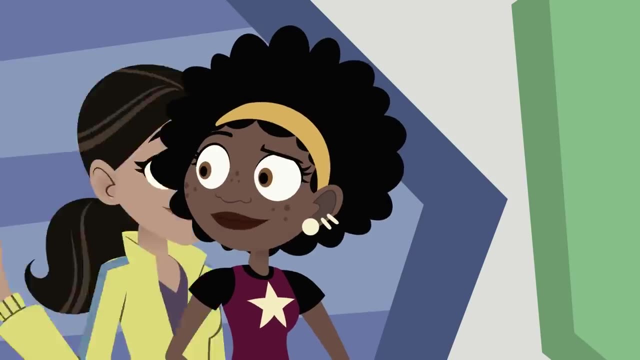 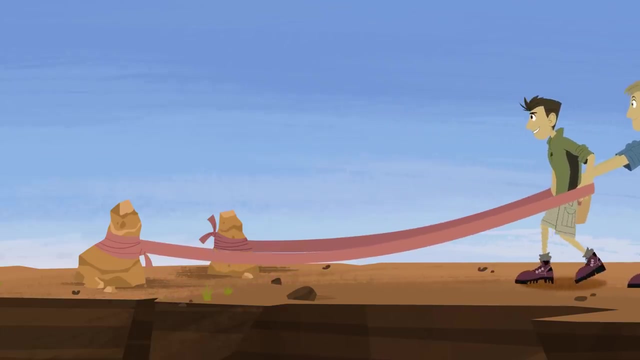 I can give you half an hour. All right, Yeah, all right. Thanks, Koki. Yeah, we'll be right back. Sure, you will. All right, this will be great. As soon as I spot the lizard, I'll let you go, and then you'll go flying after him. 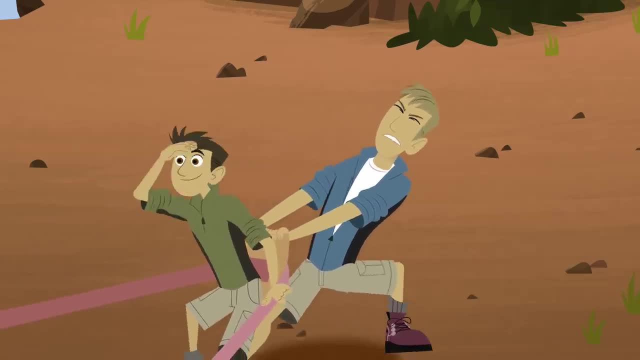 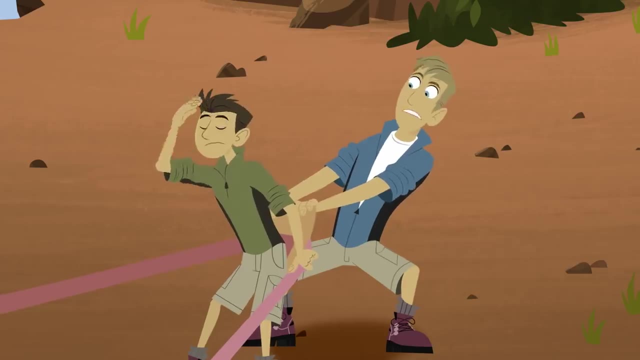 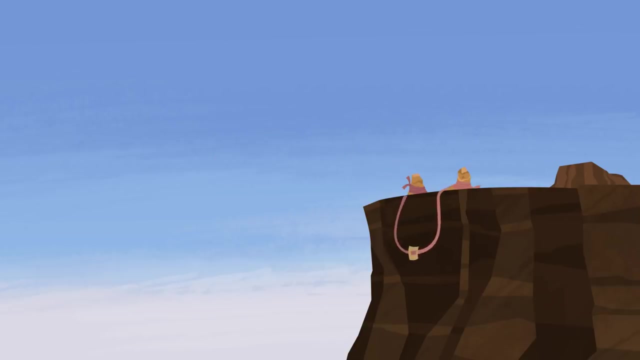 And I can grab that mystery lizard as I fly by. I should have activated bear powers or something strong. You see the lizard Not yet Could be a while. Oh, there he is. Whoa, Whoa, Ah, It's, it's, it's a. 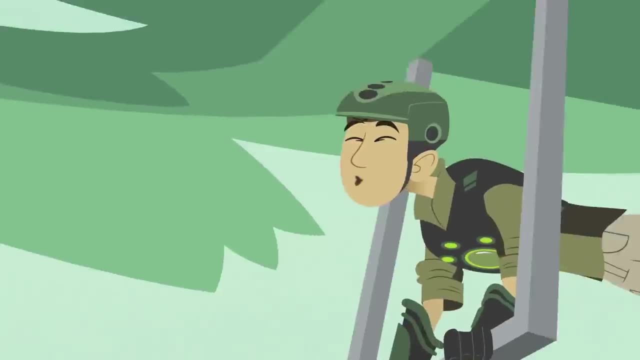 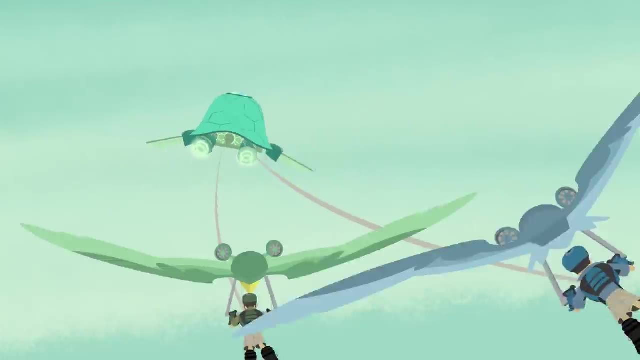 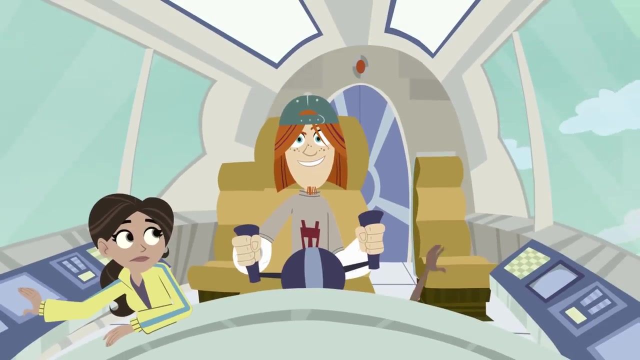 cactus, Woo-hoo, Give it all, you got. You got it. Whoa Woo-hoo, All right, Woo Woo. This is not the way to see North America. You can say that again. Smooth it out, Jay-Z, Slower. 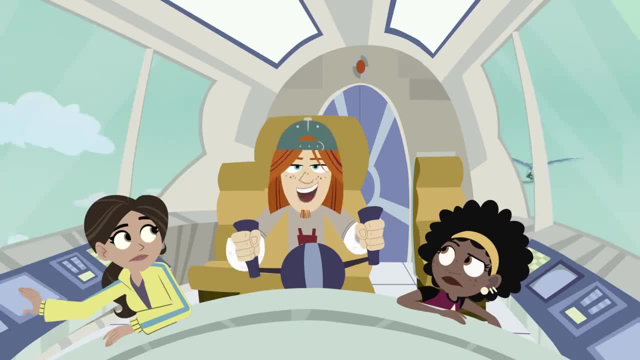 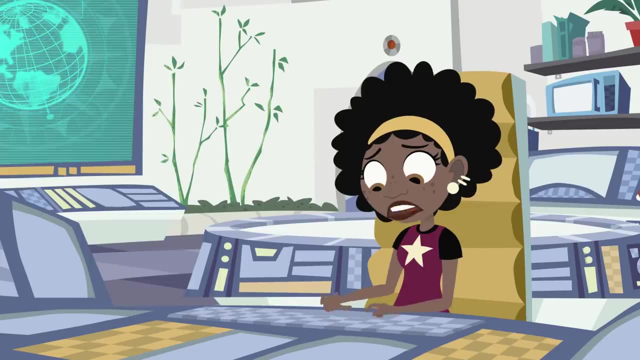 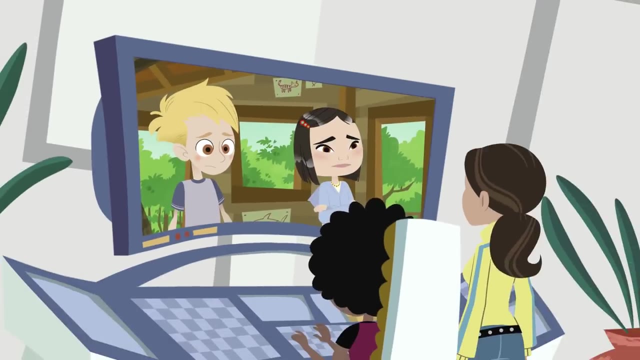 A few more turns. I'll give him the old Jay-Z jigsack, A creature alert Coming in from the north, From some Wild Kratts' kids um in eastern North America, Wild Kratts' Tortuga HQ. Mystery discovery or rescue. 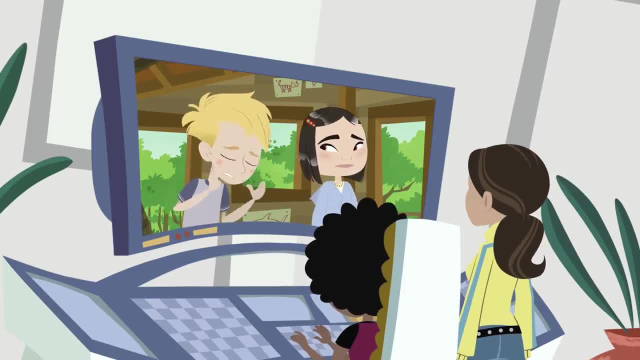 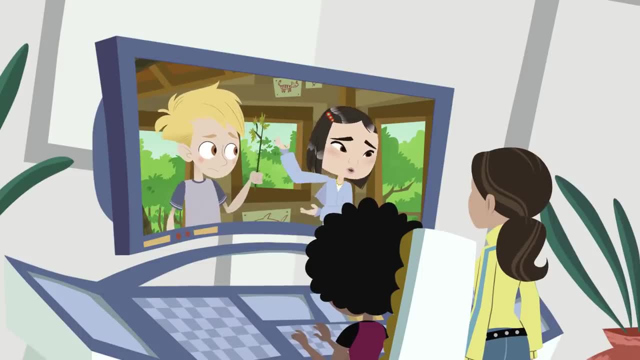 Mystery, I guess. Wait, no rescue, Wait, maybe all three. Wow, what's going on? We've got a big problem. Our clubhouse tree is dying. Even worse, The whole forest here is dying. What? All the trees are dying. 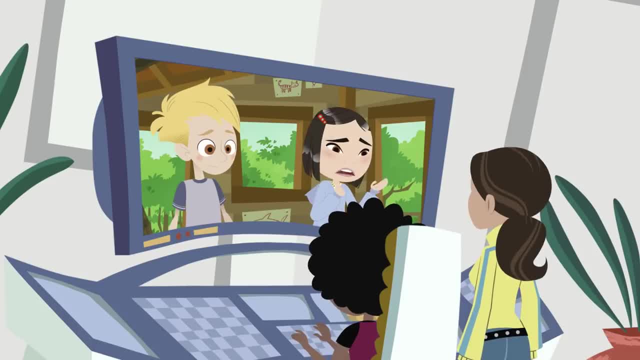 Why We don't know. We're worried about all the creatures that live here too. They can't live without their forest. See, It's a mystery and a rescue all rolled into one. We need help. You're not kidding. 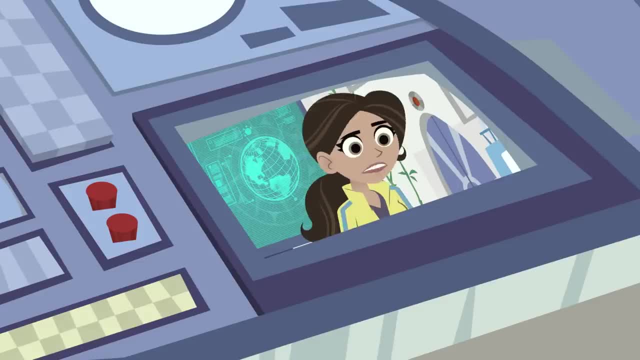 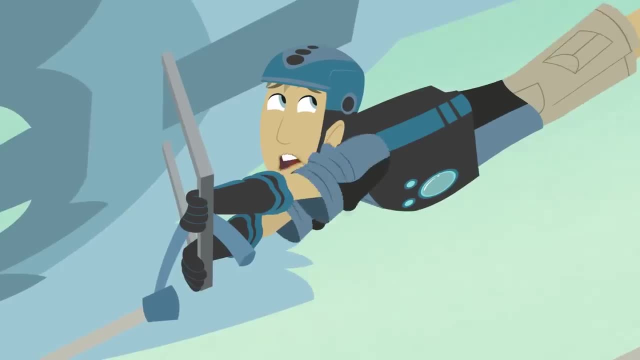 Hang tight, we're on our way. Timmy, take her down double speed. What's going on, Whoa? Did you tell him to give it all he's got? I didn't know he had this much, Whoa. 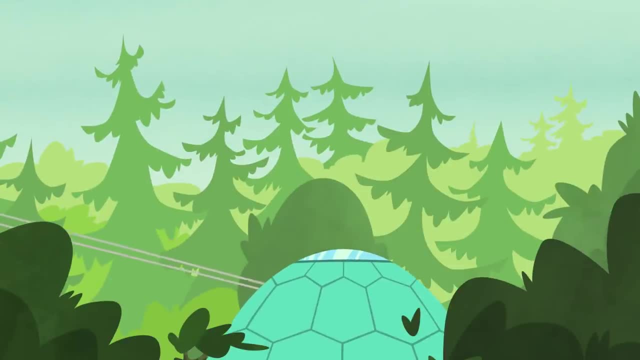 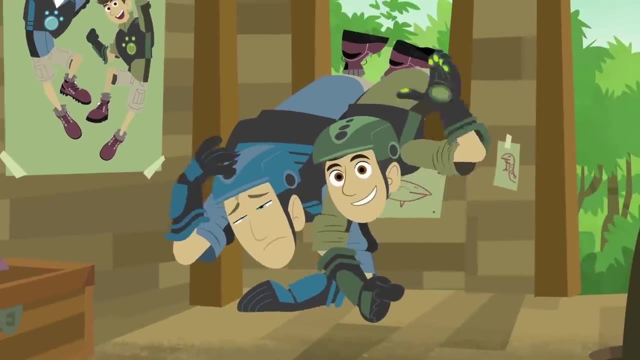 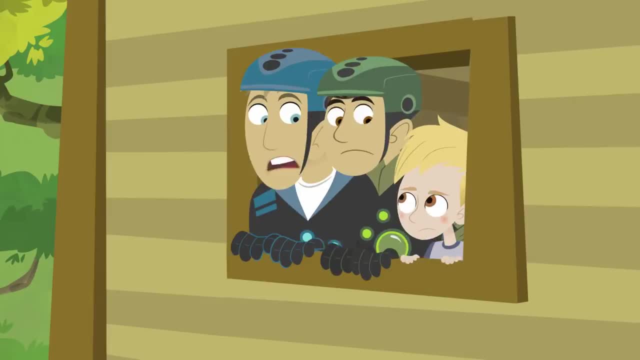 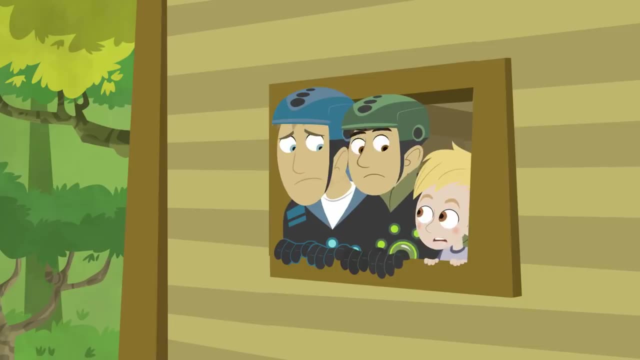 Boy, are we happy to see you guys. Oh yeah, What's up? See, it's the trees. They're losing their leaves in the middle of spring. They're sick and we don't know why. Wow, Not good. 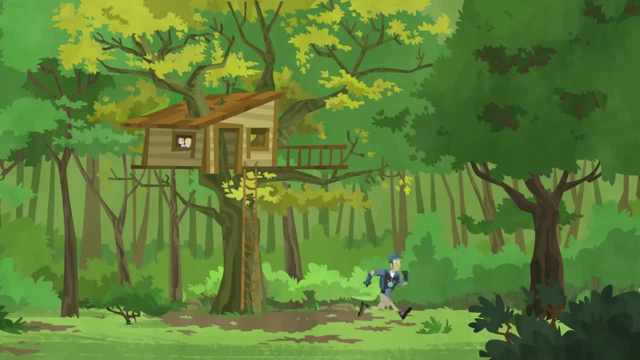 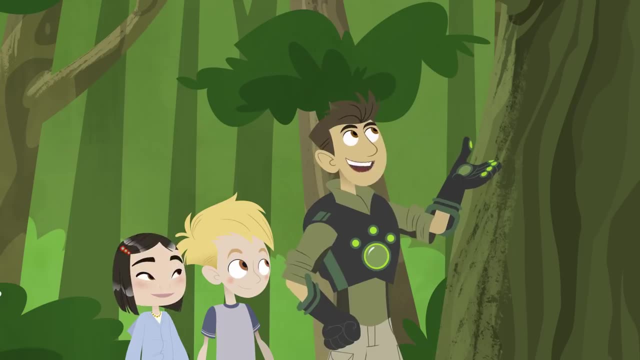 Thanks for the alert, Aiden. We're on the case. We'll figure it out. Okay, first we've got to inspect these trees. I'll do a check up top, with a little help from this guy. Activate Squirtle Power. 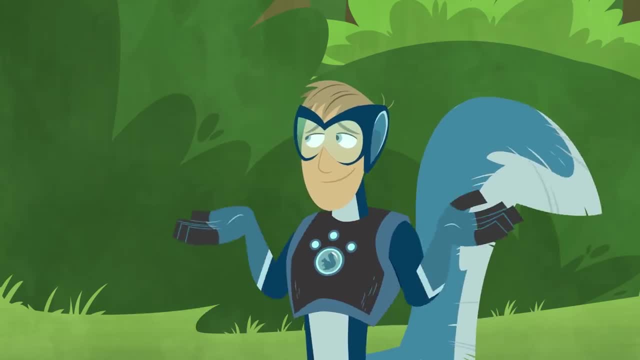 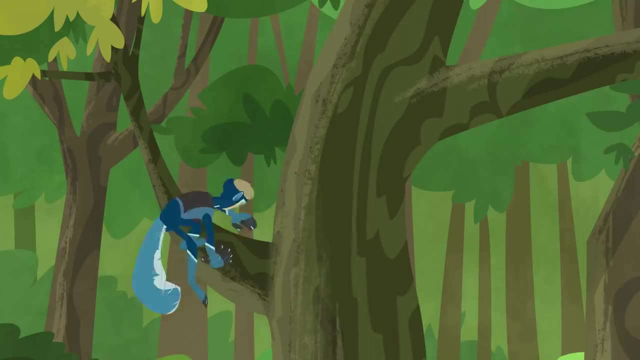 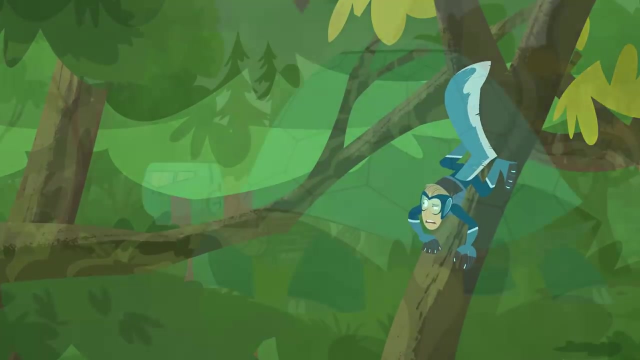 Ready to climb. Hmm, nothing unusual here on the trunk, Nothing strange here Or here Or here. So if I zoom in on the live satellite image feed, I can see what's going on with the whole forest. Wow, that's a lot of sick trees. 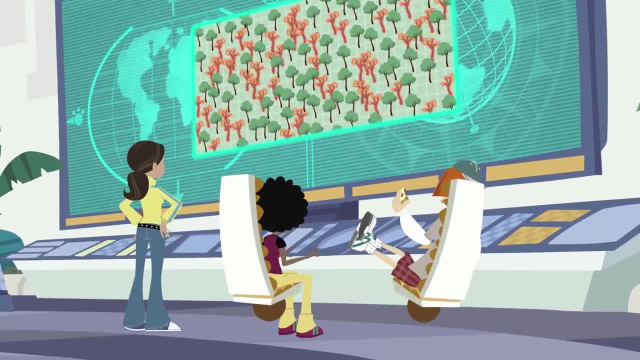 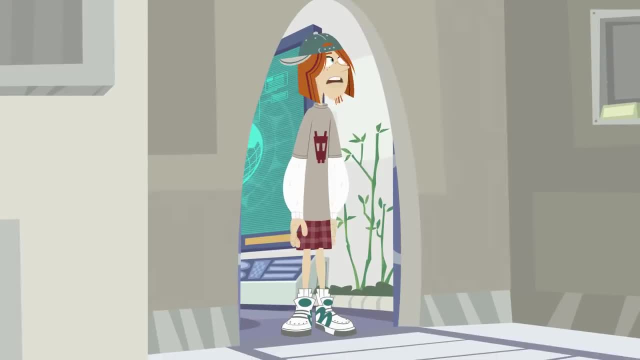 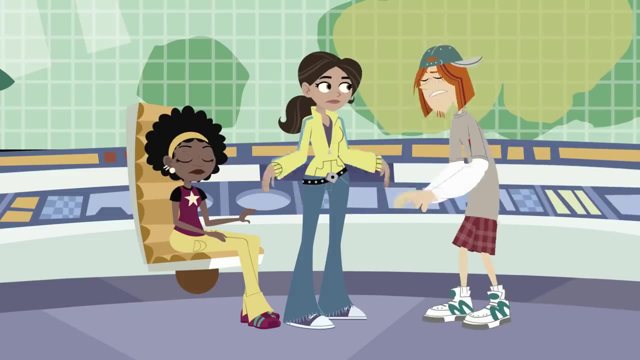 Got it Yellow? Hello, Hello, Hmm, no one there. Oh, there's another one. Oh, there's another one. This place is getting pretty weird. This place is getting pretty weird. I guess it was just the wind or something. 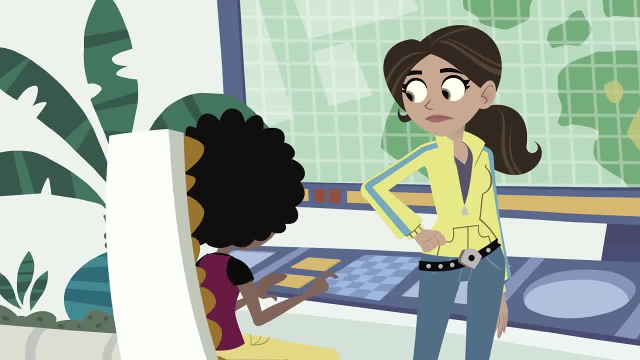 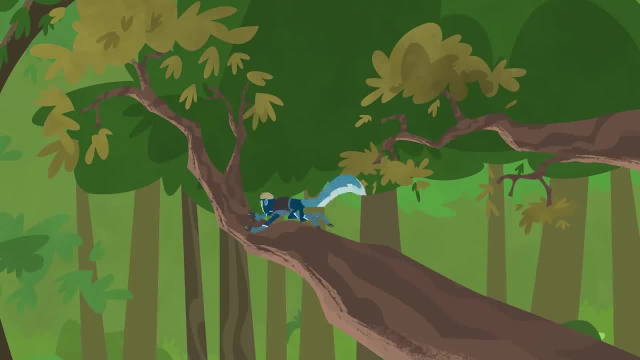 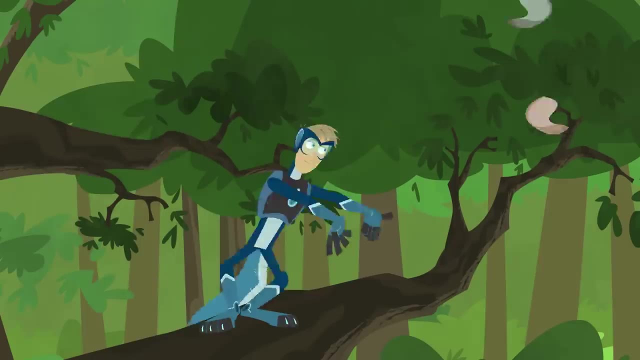 The wind knocking at the door. Yeah right, Anyway, let's get back to the tree mystery. So where were we? Yep, everything normal here And here. Whoa Back up, You found something, Seeds What. 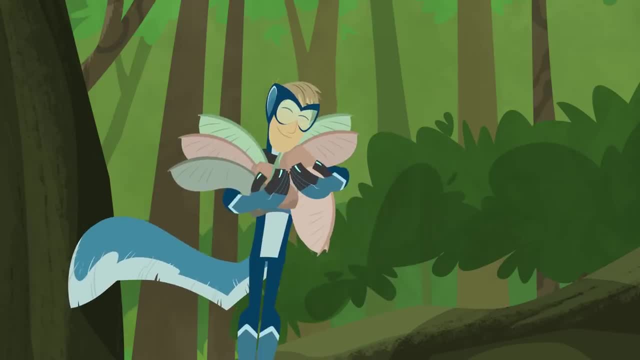 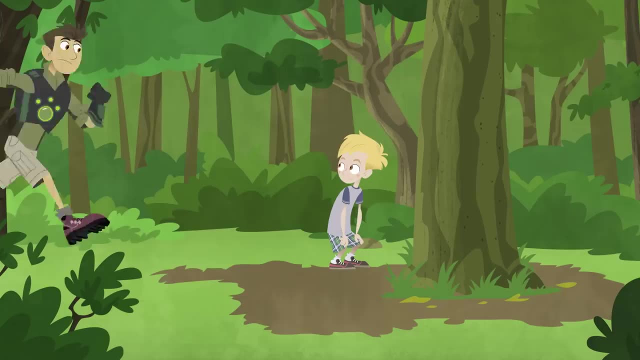 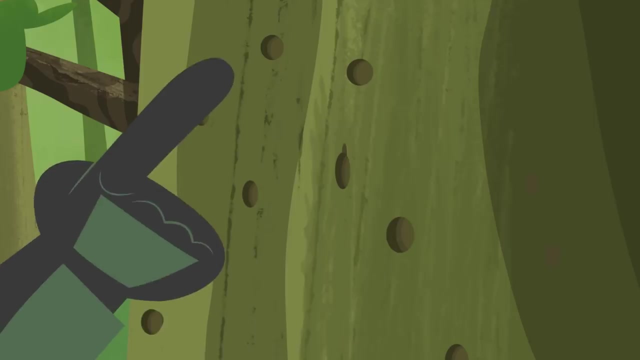 That doesn't help. I don't want you to get distracted by seeds and acorns, But stay focused, bro Right, Hey, look at this. Is this normal? No, definitely not Good spot. Small holes in the tree. 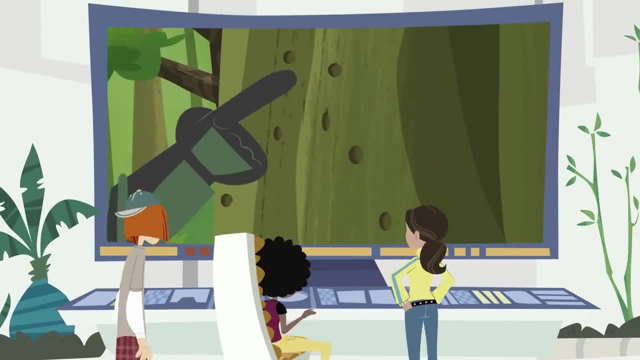 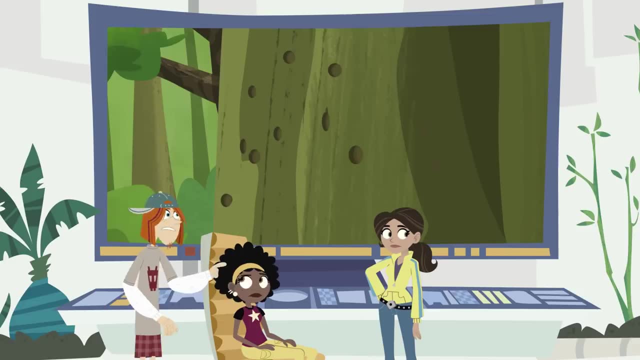 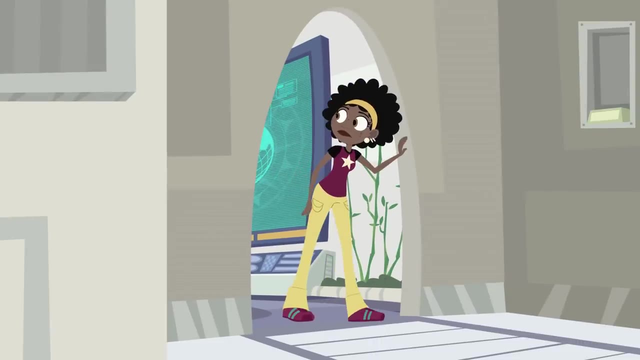 We just may be onto something here. Holes in the tree, But where could they have come from? Do I look like an expert on tree holes? There's that somebody. again, I'll get it this time. Hello, Hello, Listen, here you. 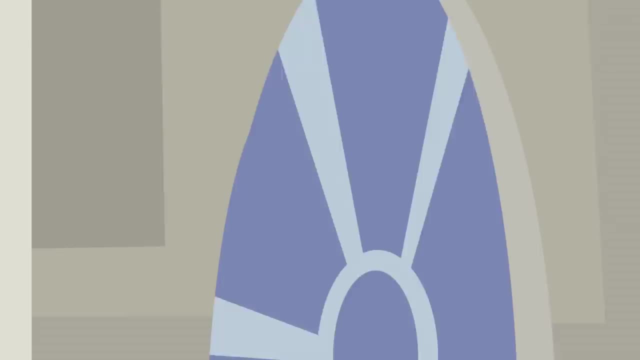 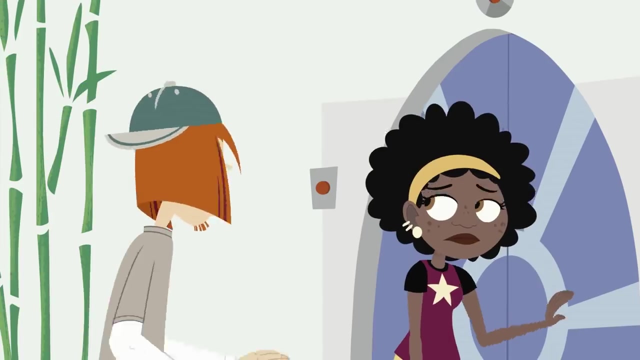 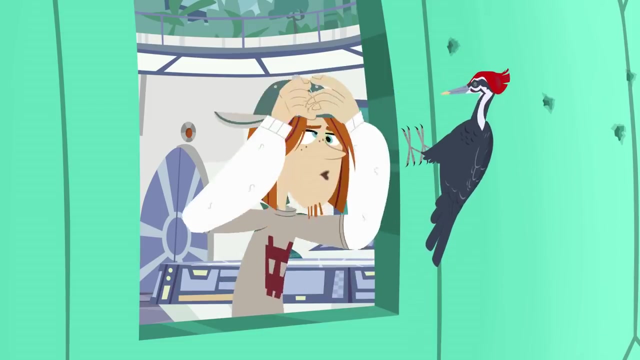 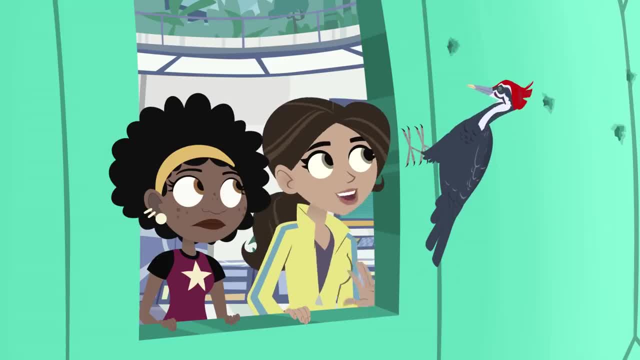 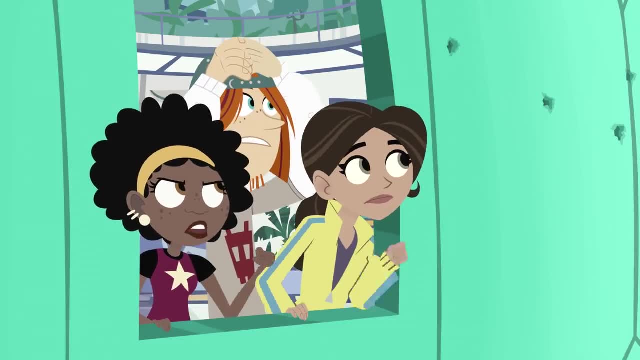 Ah-ha, A woodpecker. You're the one making all those holes in the tree. He's making holes in my forehead too. He's making holes in my forehead too. Hey, come back here. Hey, come back here. 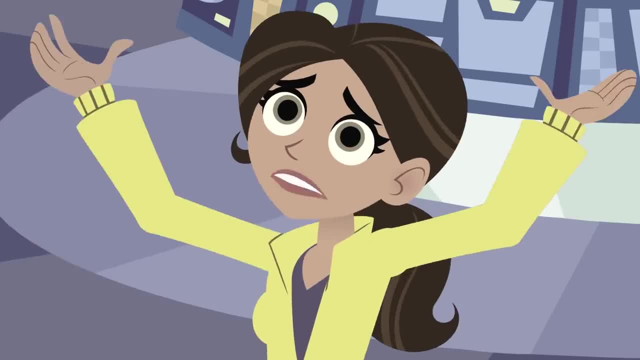 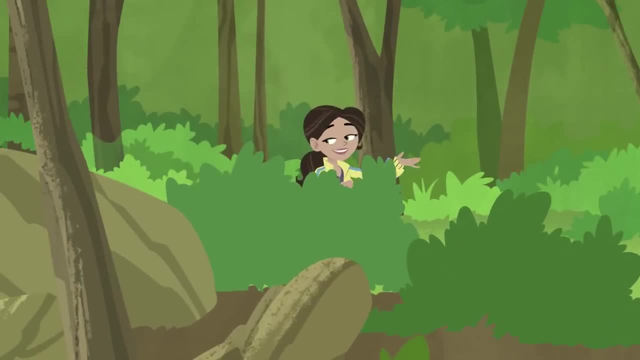 Guys, come quick. We found the mystery tree driller. We've got to stop him before he gets away. Hurry See, There he is. Oh a pileated woodpecker. Oh a pileated woodpecker. 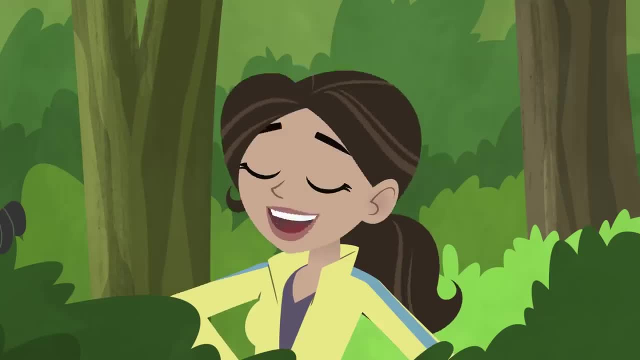 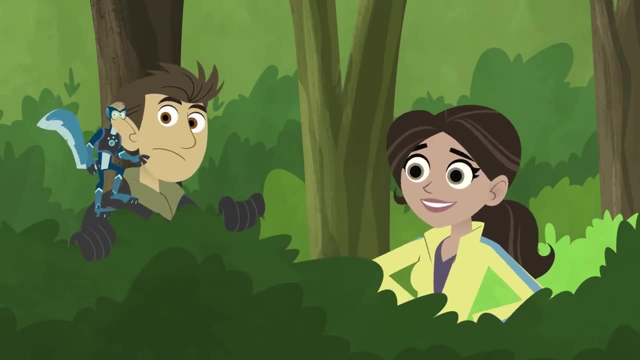 Hmm, And you think he made all the weird holes in the trees? Yep, he's the culprit. I mean, did you see him do it? Well, he made one at the door of the Tortuga And almost made another one right here in my forehead. 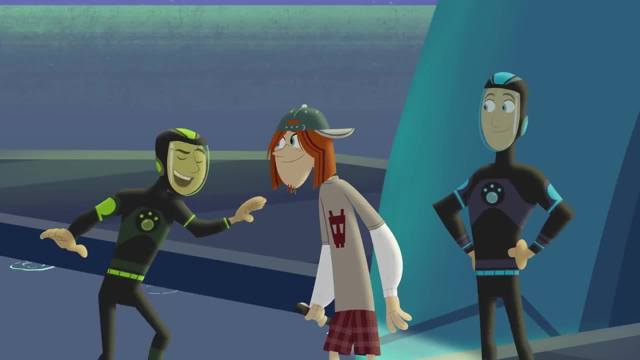 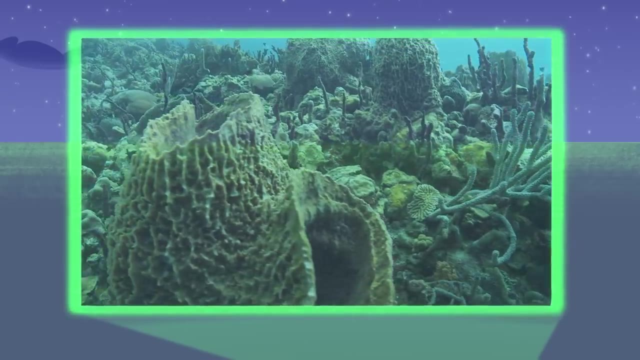 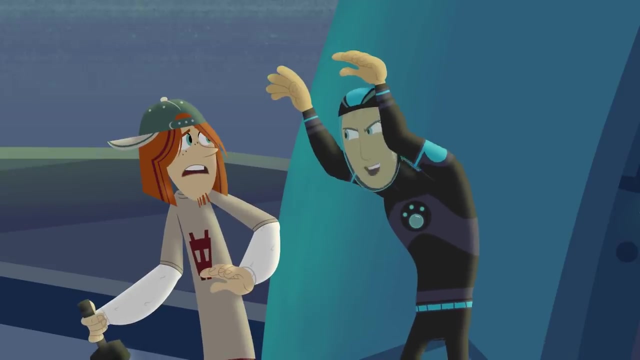 And almost made another one right here in my forehead, Jimmy. the creatures we're heading down there for are very strange sea creatures that built the coral reef. A creature makes that. I thought it was rocks and stuff. No way, It all comes from an animal. 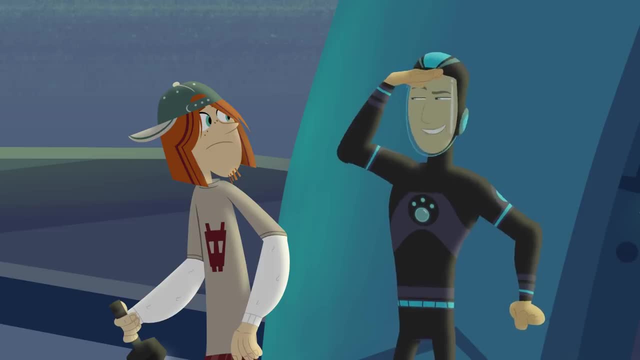 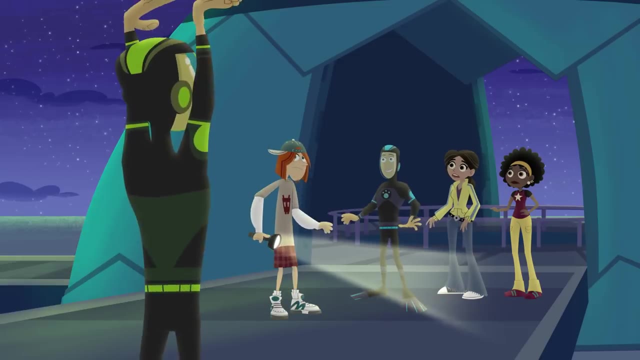 A special animal that hides out during the day. A special animal that hides out during the day And at night, under the cover of darkness. they come out and they build, Bit by bit, higher and higher. the reef rises So big it's the largest living structure in the world. 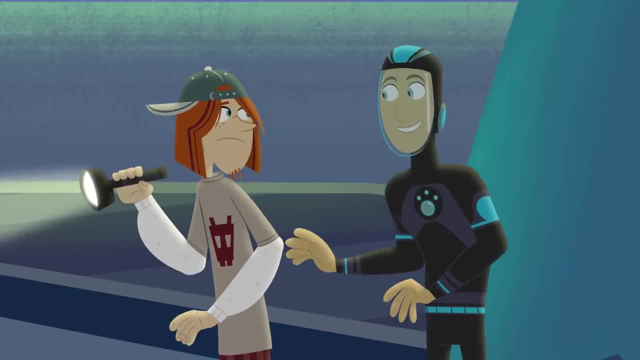 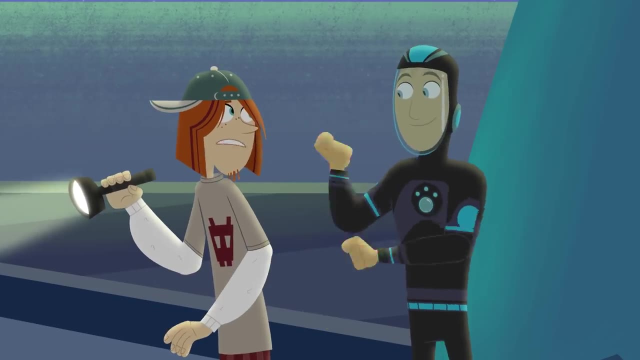 So big, it's the largest living structure in the world. But by dawn, when the sun rises, they go back into hiding Gone, Like they were never here. Okay, Are you trying to freak me out? Because it's working. 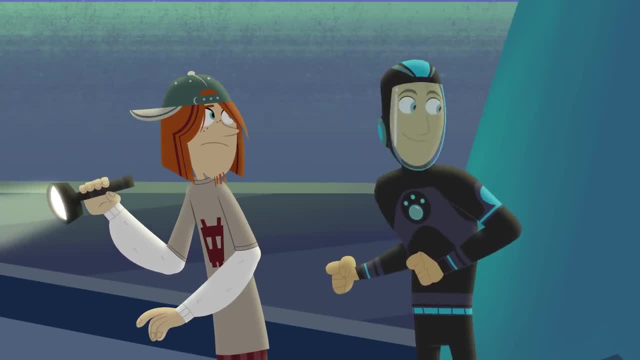 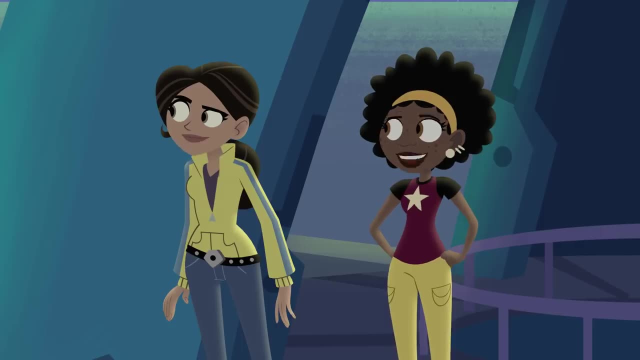 It's exciting, Jimmy, I'll say. I thought we were going down to do a checkup on reef health for the World Reef Science Team. But who are these creatures And how come no one ever told me about them? And how come no one ever told me about them? 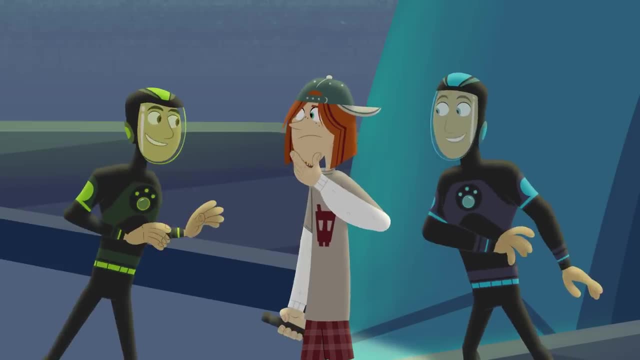 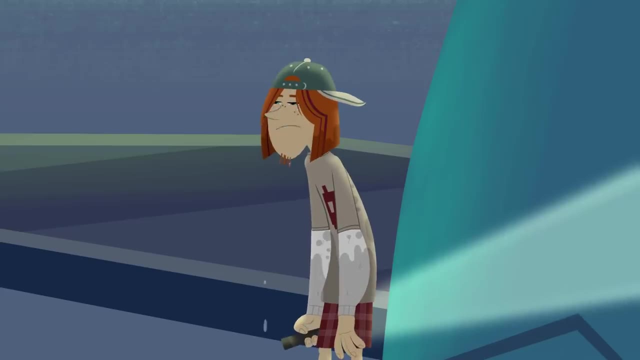 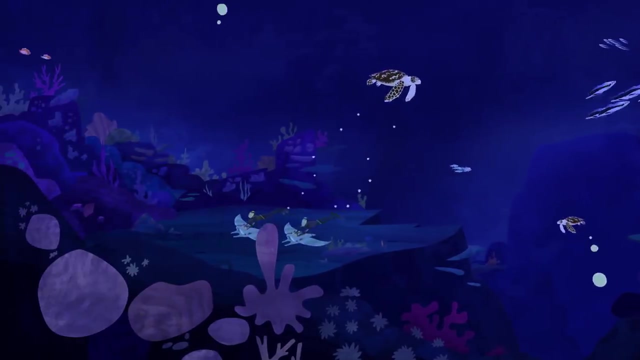 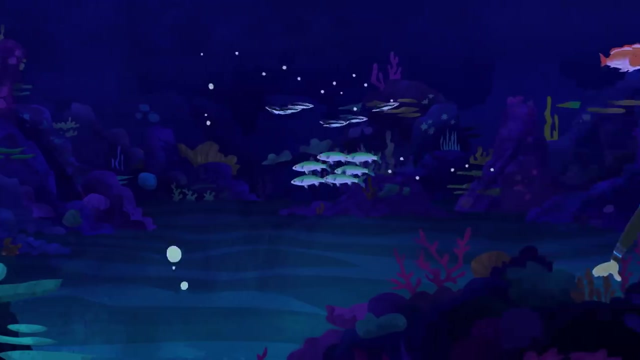 What are they called? Polyps? See, ya, See, ya, See ya. What a funny name. This should be a good spot to find the martin. Oh yeah, Oh, I hope we got here in time. Yeah, They should be coming out right about now. 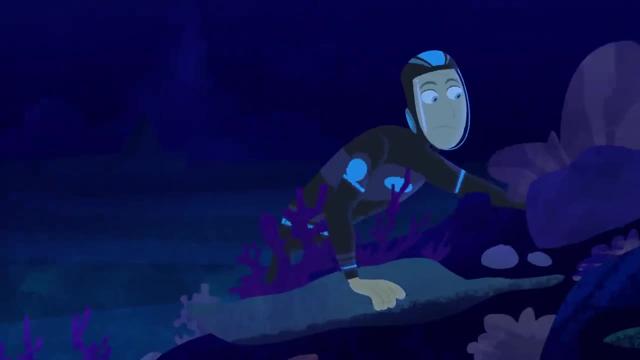 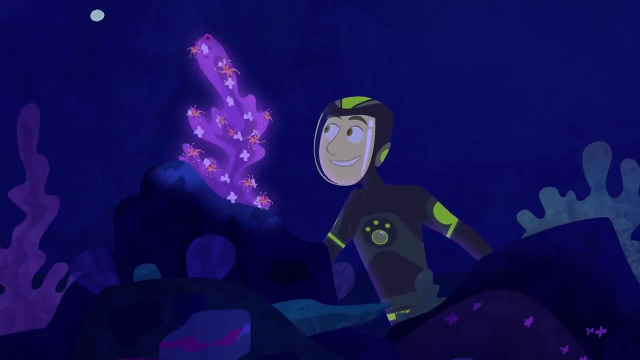 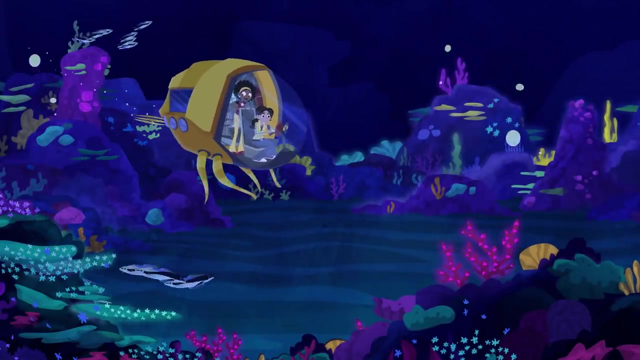 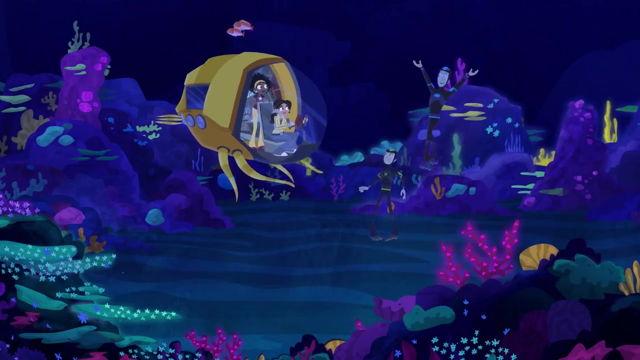 Hmm, No sign of them yet. So now we wait. Look, They're coming out. Oh, Polyps, They're everywhere. Wow, They're beautiful. You mean, these colorful things are creatures. They look like flowers. Oh yeah, They're animals, all right. 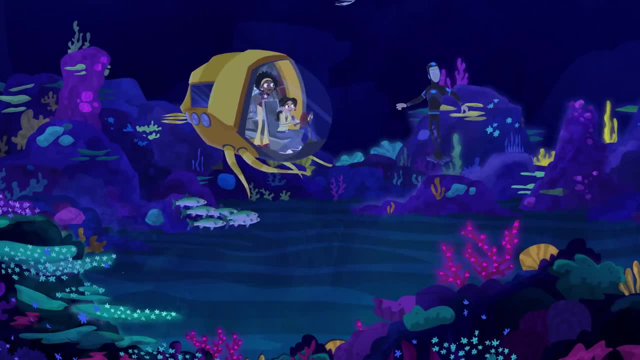 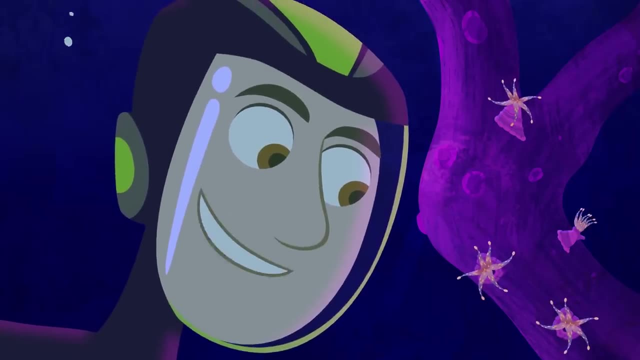 Every one of them is a creature. And check it out. The hard, rocky part is their skeleton. See, they build a skeleton outside their bodies and they can hide inside it, protect it until they're ready to come out. You mean this whole reef. 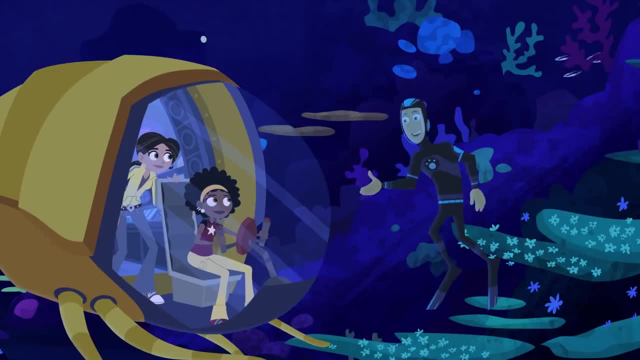 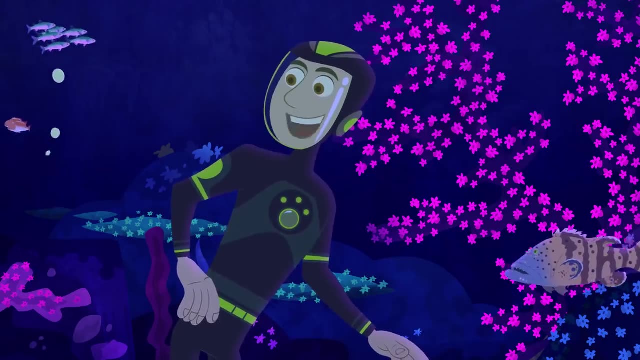 is made of the skeletons of these little guys. That's right. Polyp skeleton built on polyp skeleton, built on more polyp skeletons for millions of years. And now millions of creatures live here in and amongst the coral, More different types of sea creatures. 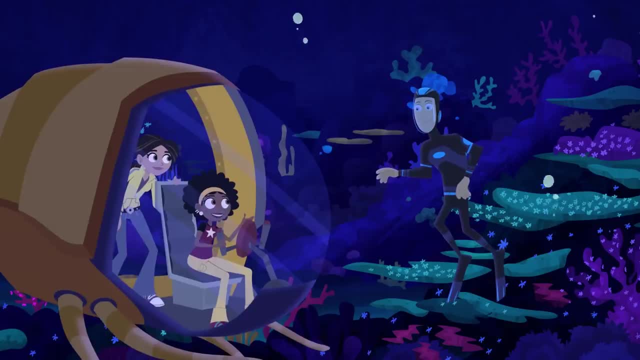 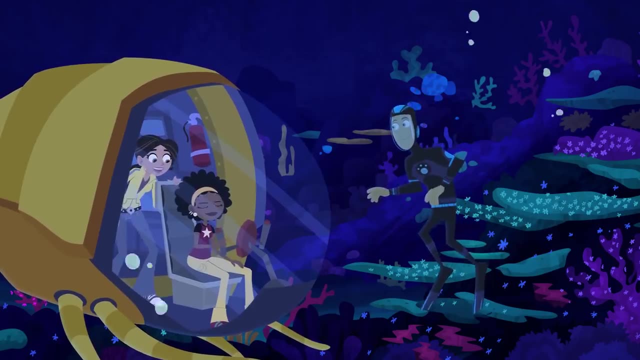 than any other ocean habitat. Yeah, but we know these reefs are fragile habitats And if we're going to do our annual reef checkup to make sure it's healthy, we'd better get to it. Okay, let's get in there for a close look guys. 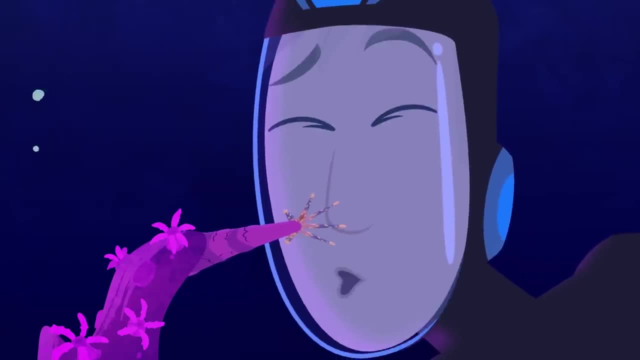 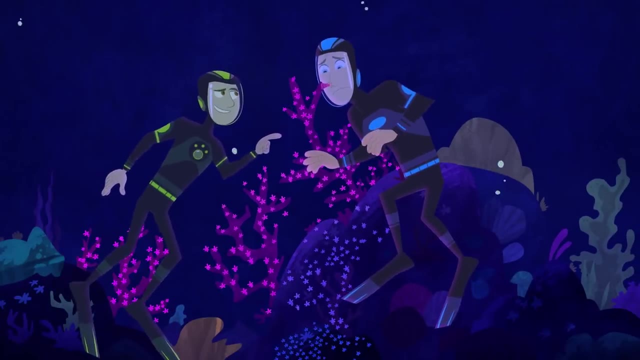 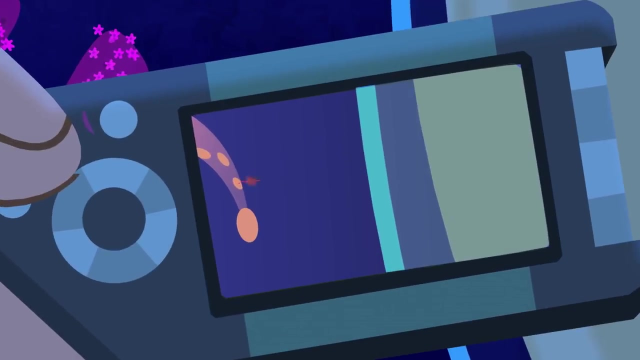 On it. Ah, Close enough. Oh, bro, You just got harpooned. What Harpooned? You have to zoom in with a microscope to see it. But the polyp shot that tiny needle-like harpoon from his tentacle. 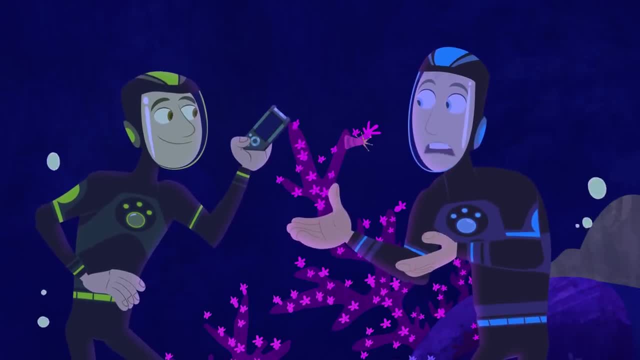 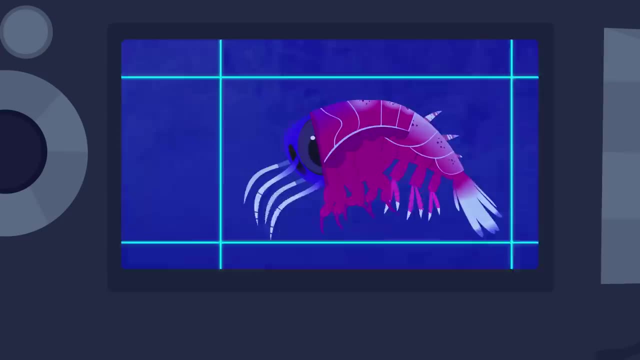 That's how they hunt for food. Hey, what are you harpooning me for? I'm not food. Ah, here comes some stuff that's probably tastier than you. Ultra zoom on. That's what they love to eat: Amphipods. 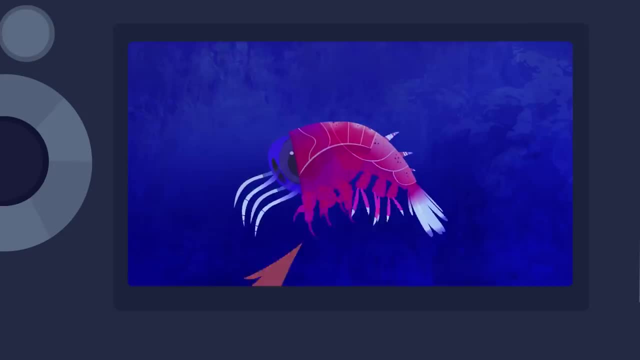 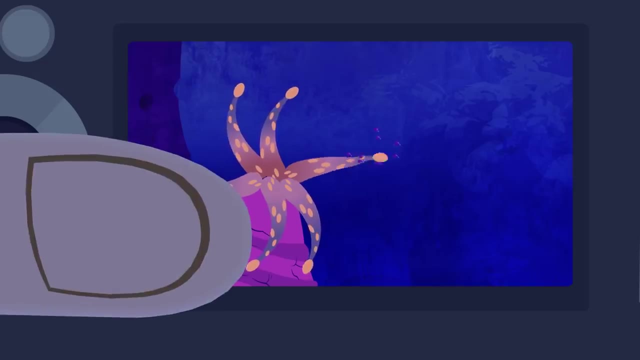 See, there are the harpoons ready for launch. Ooh, He did it. He scored some launch. He reels it in with his harpoon and the tentacles push the little meal to his mouth right down there in the center. Wow. 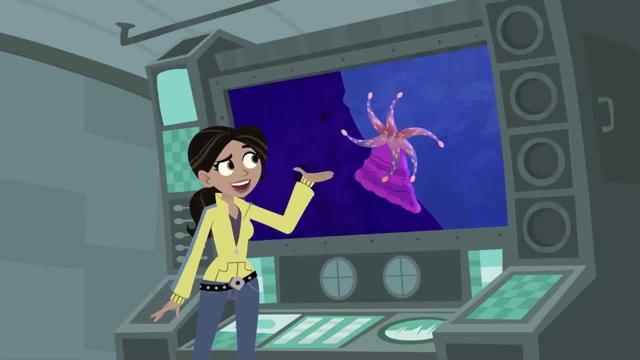 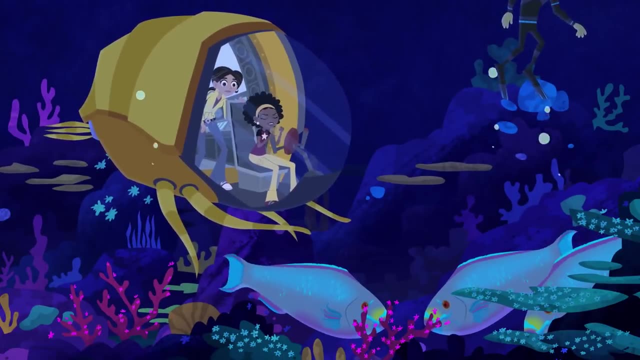 I like these little guys And all this time I thought coral was just a bunch of rocks. Hey, What are you doing? Leave that coral alone. Those fish are destroying the reef, So that's why the coral reefs are disappearing, Those reef-eating fish. 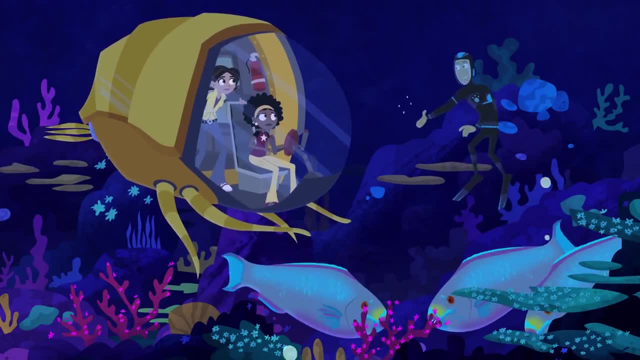 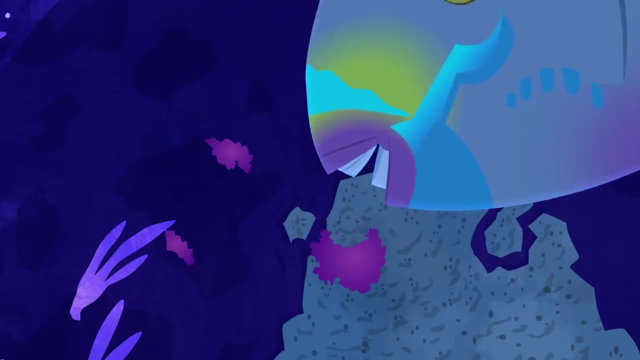 Whoa, They're fast. They're parrotfish, Aviva, and they're not why the reefs are in trouble. Check it out. He's scraping algae off the coral with his hard beak and eating it, And he does kill and even eat some polyps while he's at it. 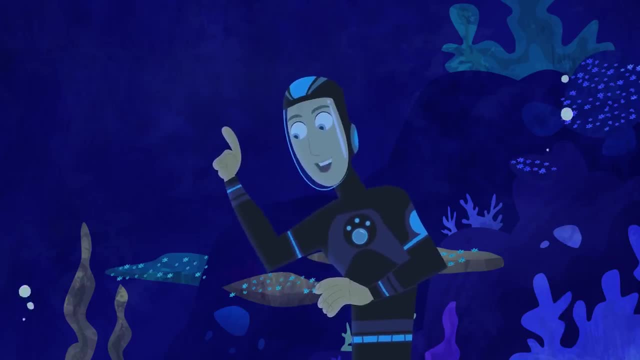 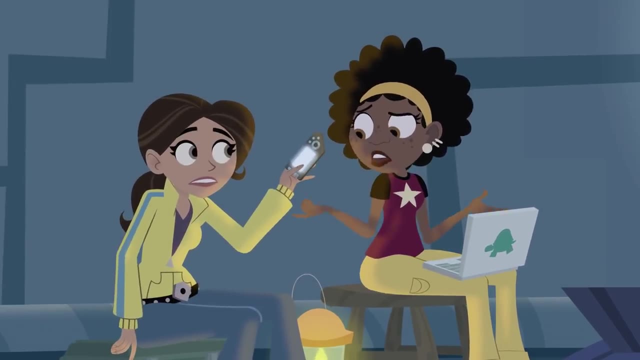 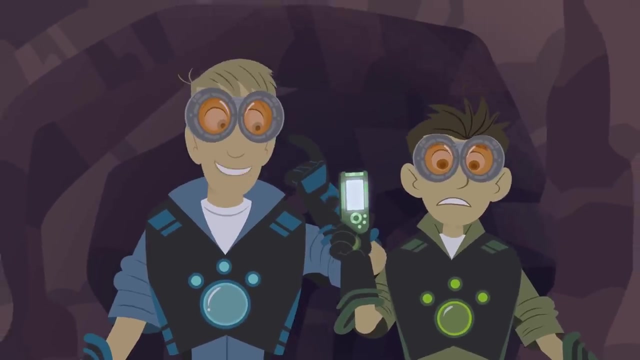 But he's also keeping the algae from taking over and choking out the reef. Hello, Hello, What in the world? Where on Earth are you guys In Earth actually? Yeah, we're taking a new approach to our search. We're seeing with heat vision. 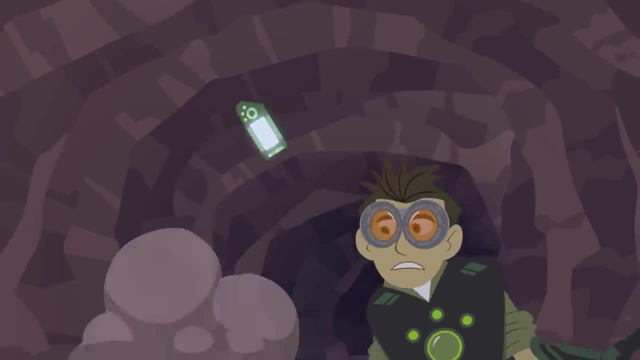 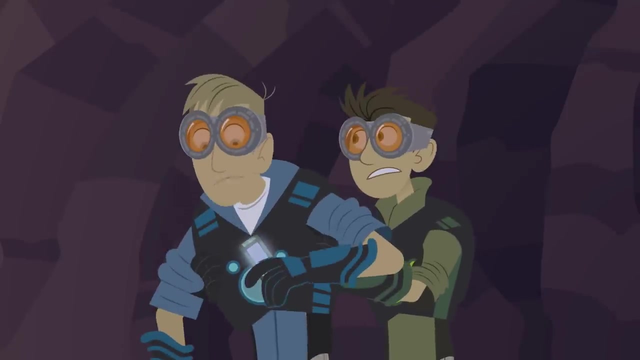 and walking around through the tunnels of ground, squirrels walking behind a rattlesnake and Uh, the only problem is pebbles on the ground don't give off heat, So we can't really see them with heat-seeing goggles on. 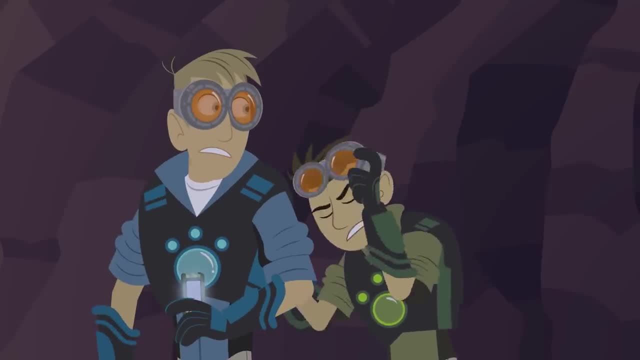 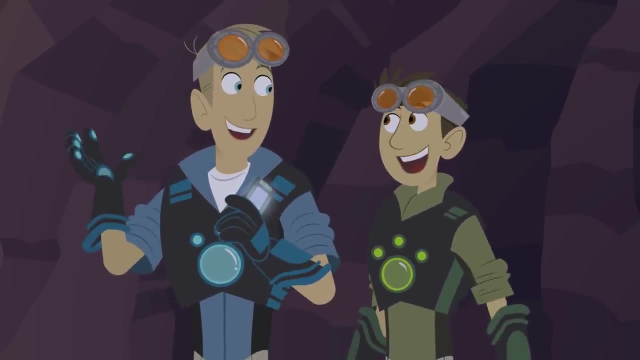 Wait a sec. If we can't see the pebbles that are tripping us, then we won't be able to see the tellurium crystals either. We need to see with heat and with our eyes. Uh, Aviva, We need rattlesnake power, sir. 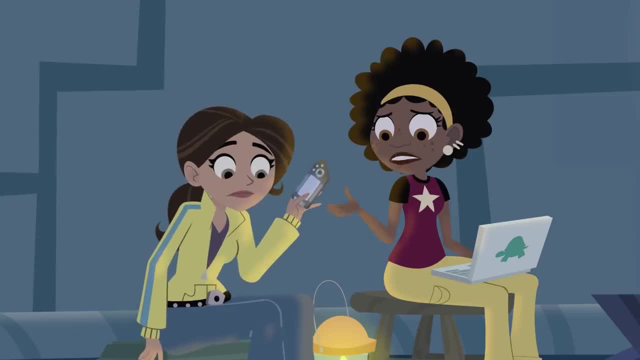 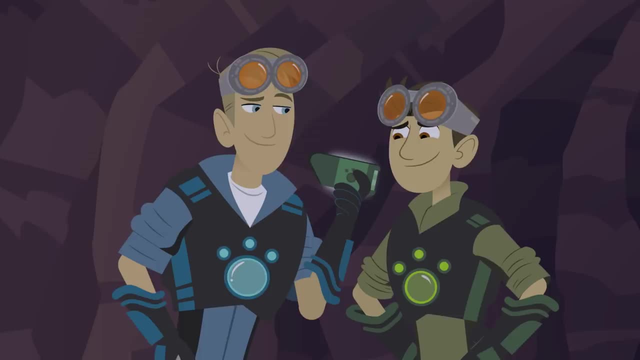 That would not be a good idea. Creating one power disk would suck up the remaining power. And remember, tellurium is very rare, Even with rattlesnake powers. there's no guarantee you'll find it. Oh, but ground squirrel burrows. 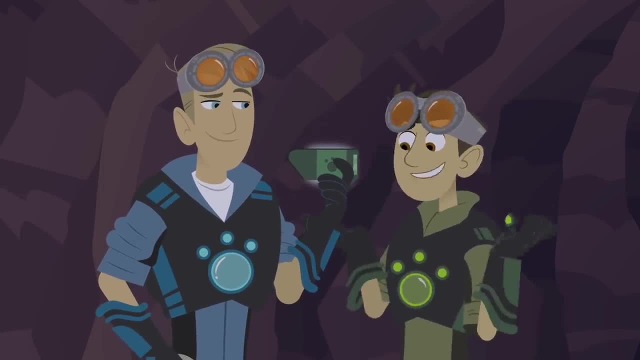 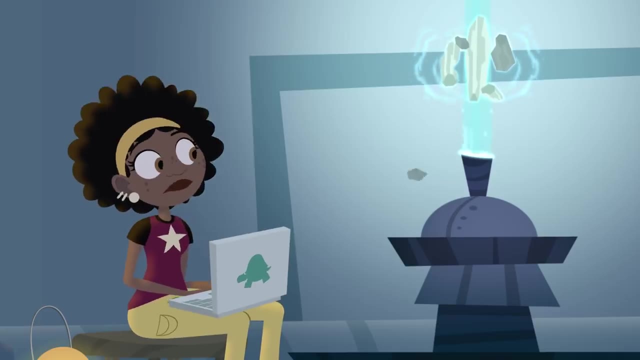 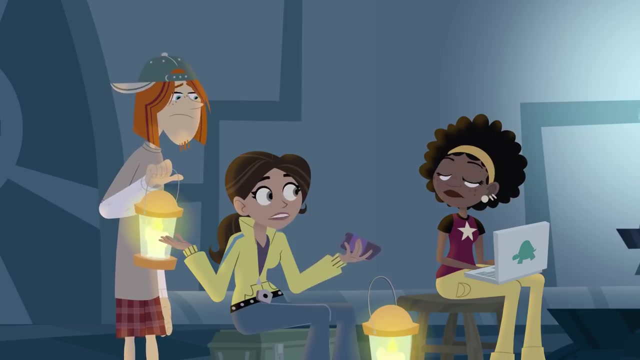 are extensive. in the Sonoran Desert Alone they cover thousands and thousands of square kilometers. Of course we'll find tellurium And we've got to do something. If we don't find tellurium, our core will fade out in just two hours anyway. 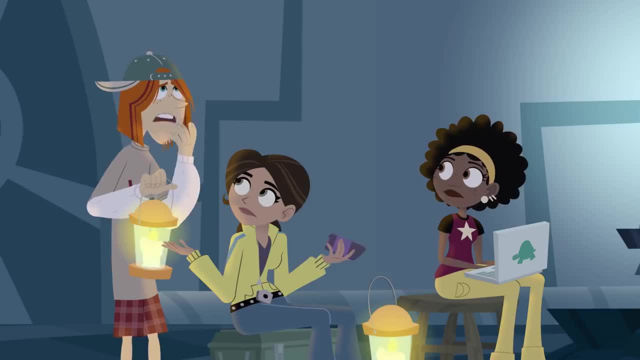 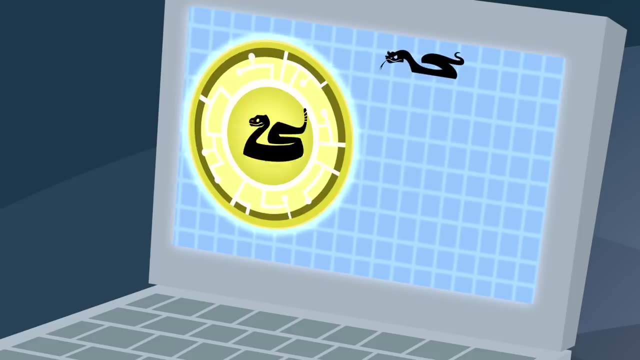 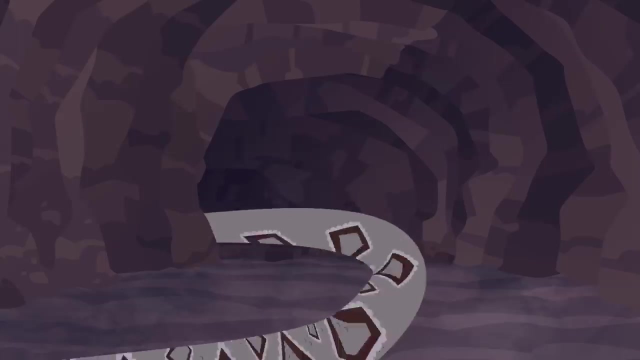 We've got to try. We do kind of have to try. We've gotta try. I'm gonna start modifying the eyelash viper disk with rattlesnake powers. Yeah, these rattlesnakes' long, thin body design. lets them go. 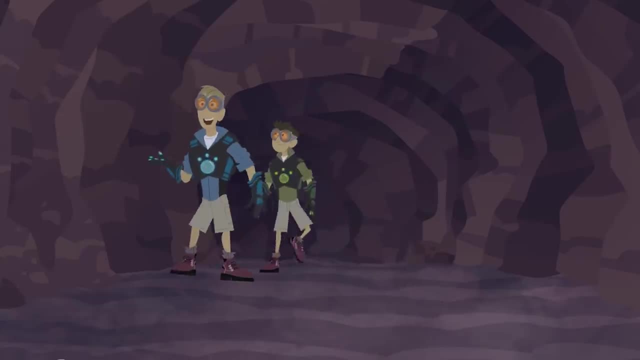 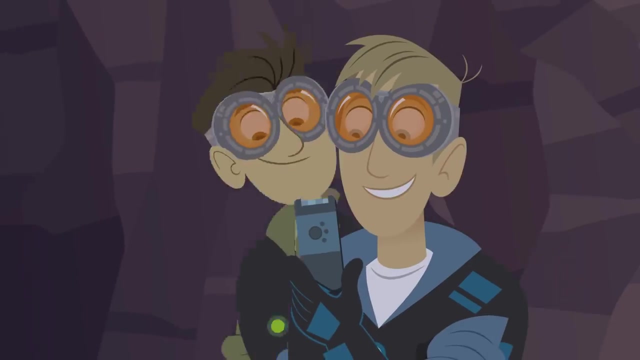 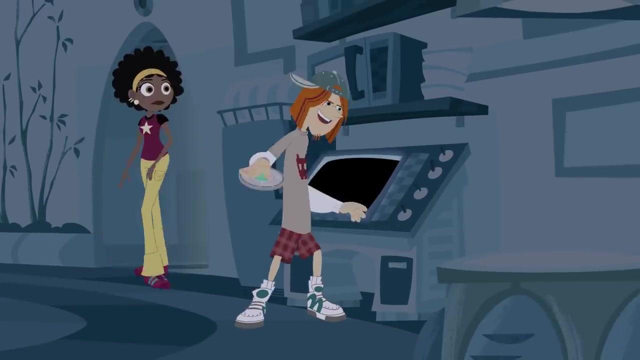 anywhere in the ground squirrel tunnels. He's just looking for a spot to set up an ambush. Hello, Martin, Chris, I'm done. The rattlesnake power disks are ready. Jimmy Cat Energize and Jimmy no. 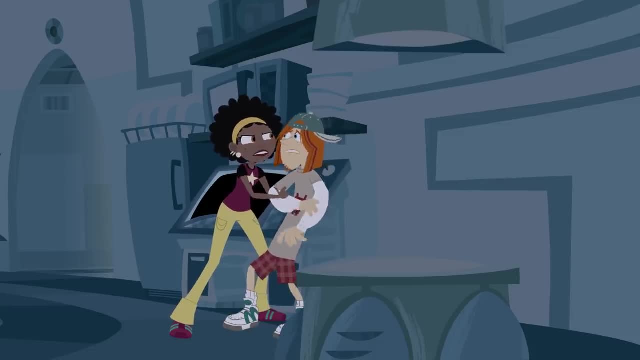 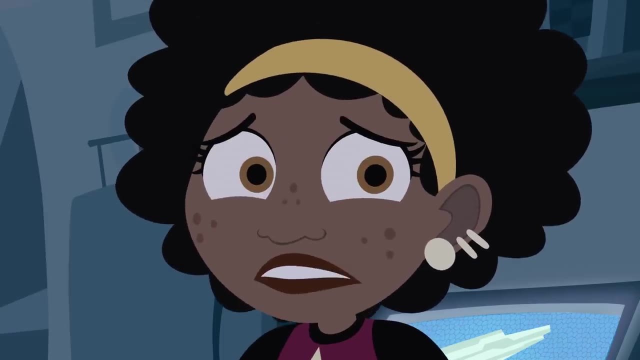 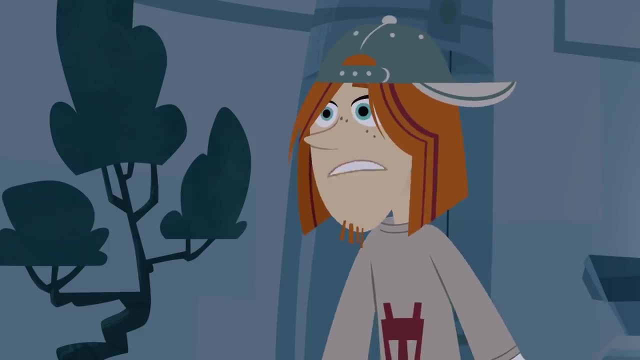 We didn't have enough power for teleportation. Sorry, I forgot. We've got 30 minutes And then an irreversible meltdown begins. We'll be totally dead. But then how are we going to get the miniaturized rattlesnake power disks? 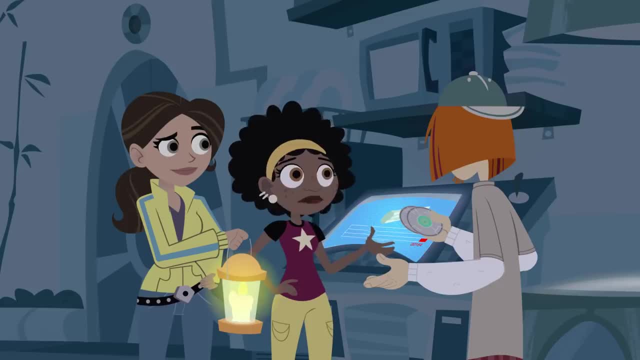 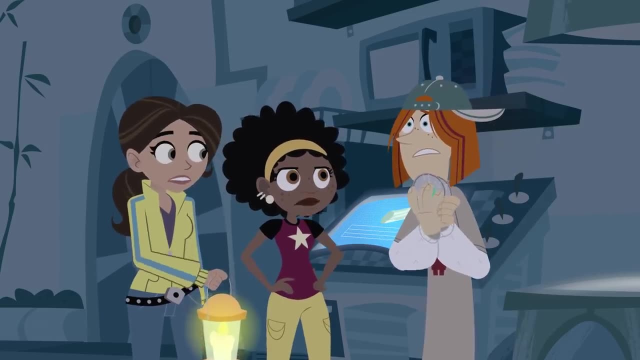 to the Kratt brothers so they can find the tellurium. Jimmy, you'll have to deliver them by hand. What He looks snakebitten. Maybe that's what he's worried about. Jimmy, it's your job to teleport the disks and we can't do that now. 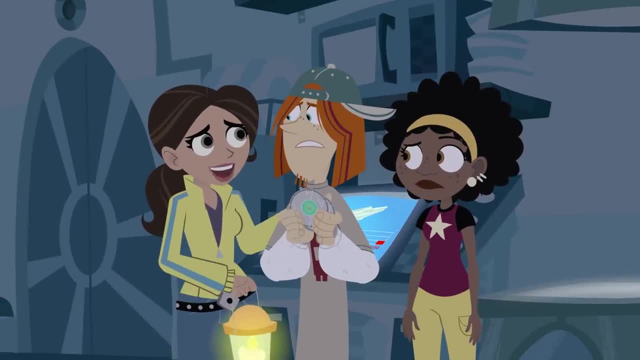 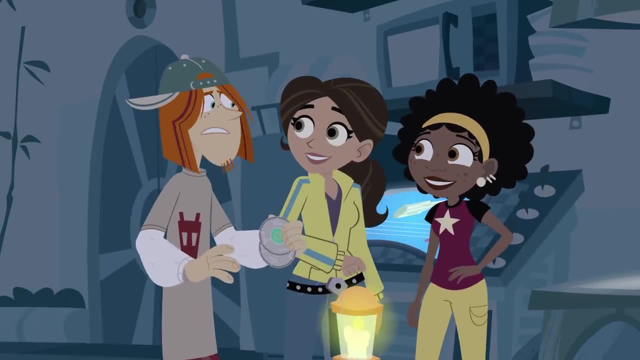 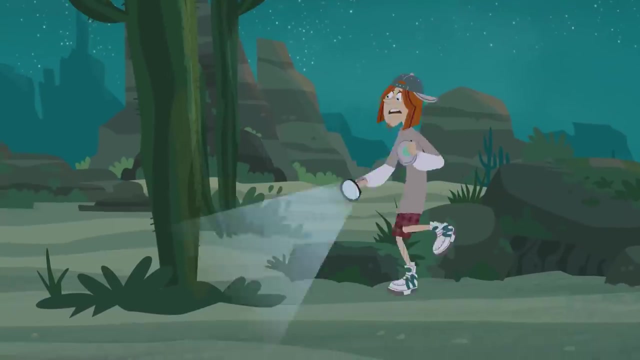 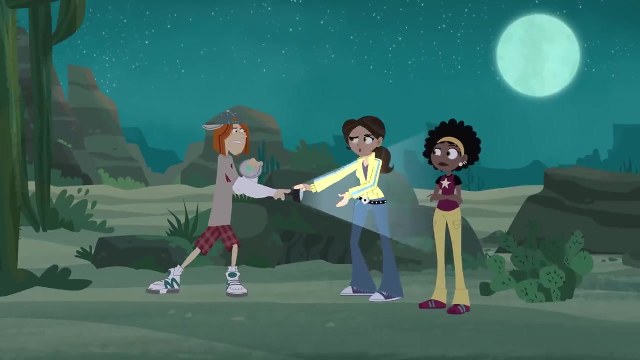 So you've got to hand deliver them. Come on, Jimmy, you can do it. Okay, Yeah, I can do it. Yay, Woohoo, All right. Uh, Jimmy, That's just a saguaro cactus. 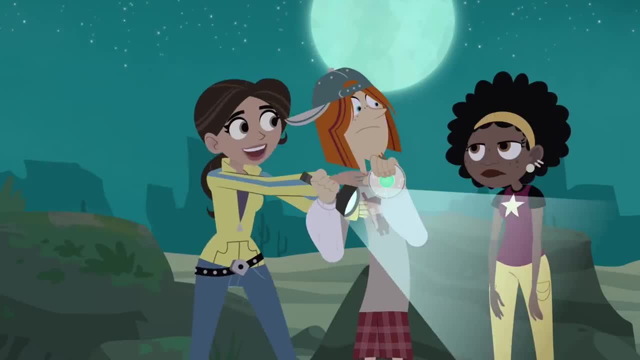 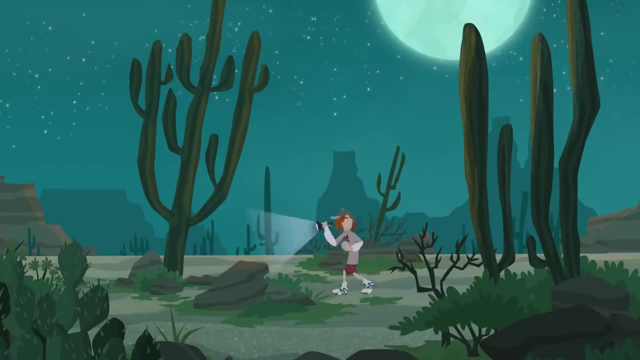 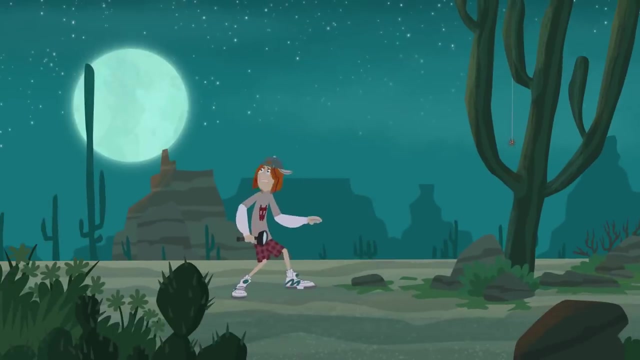 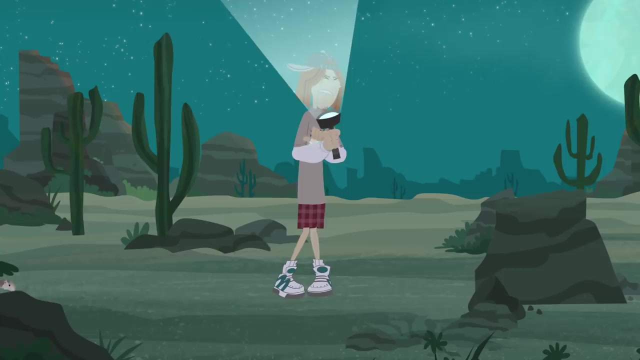 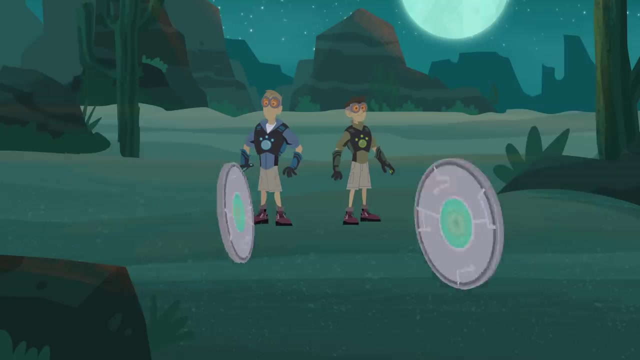 Oh, I knew that. Okay, Jimmy, keep going. Oh, Oh no, Oh my, Hey, Jimmy. Ah Nice, Chris Marta, Perfect timing buddy. Thanks, Jimmy, Y-y-y-you're welcome. 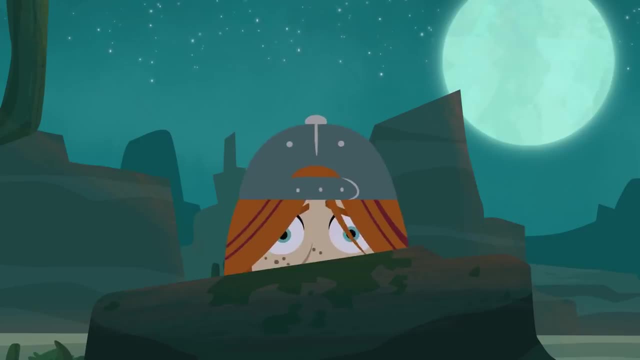 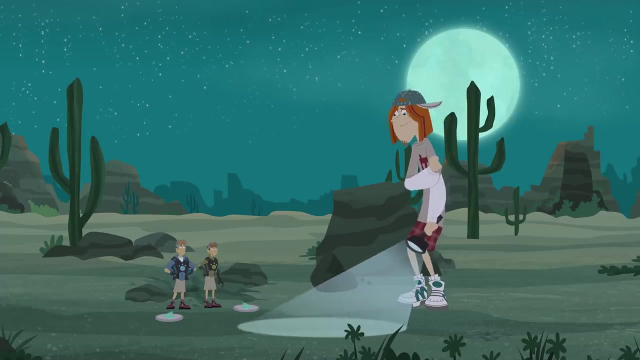 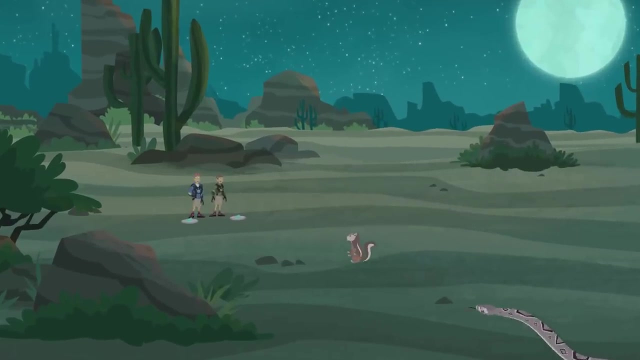 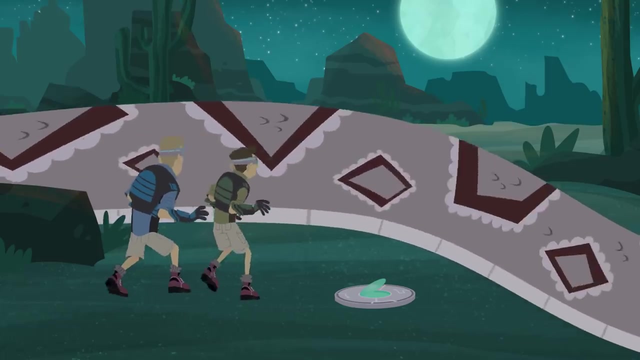 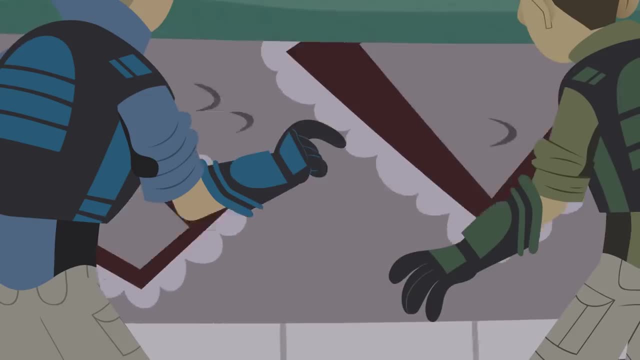 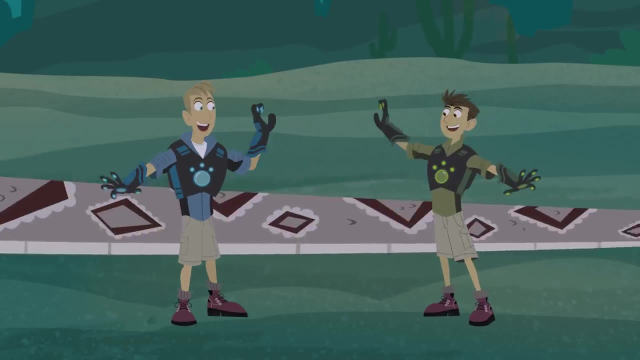 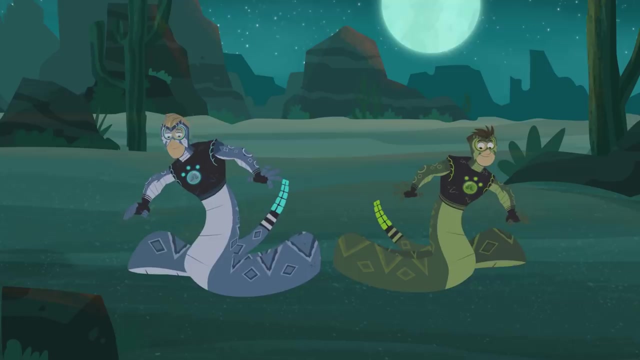 Rattlesnakes have big rough scales. Oh, check out this pattern. See the diamonds. That's why this species is called a diamondback rattlesnake. Activate creature power suits Rattlesnake powers. Hey, let's get underground.